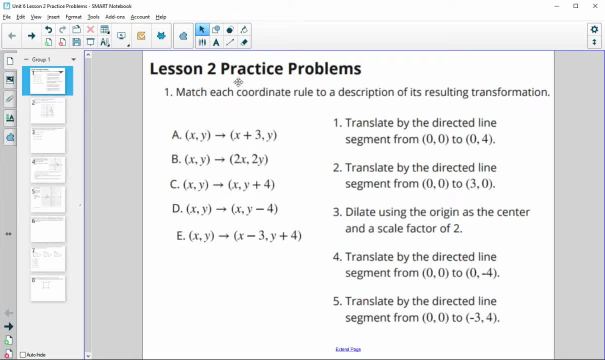 Let's take a look at lesson two, practice problems from unit six. So this one says: match each corresponding rule to a description of the resulting transformation. So some things to look at here. what I would look for is some key words and match those two possibilities. So here, 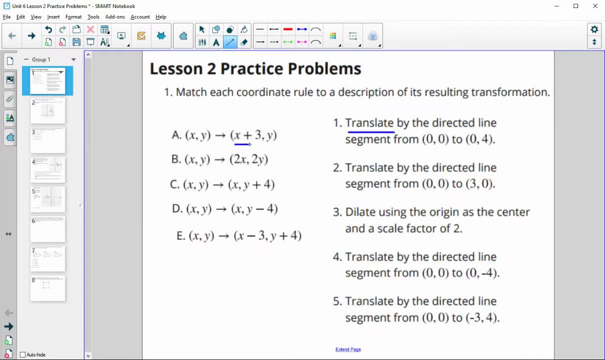 I see translate and translations look like this, with addition or subtraction in them. So I know that each of these is a type of translation, so that rules out B for me. So all of the rest of these say translation in them. So the only one that doesn't say translation is number 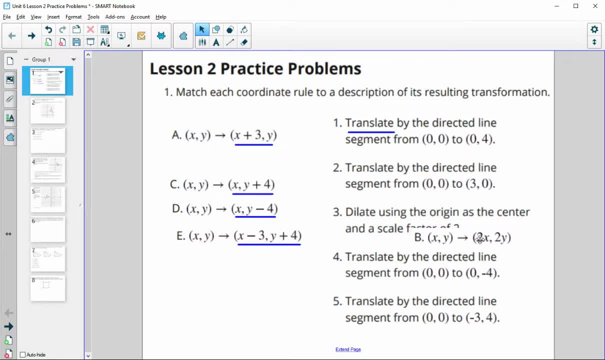 three. So this one is a dilation and we know that because of the multiplication, So B goes with number three. So dilation around the origin by a scale factor of two, So B matches to three. And then you kind of want to match these translations, what they're doing, to the X and 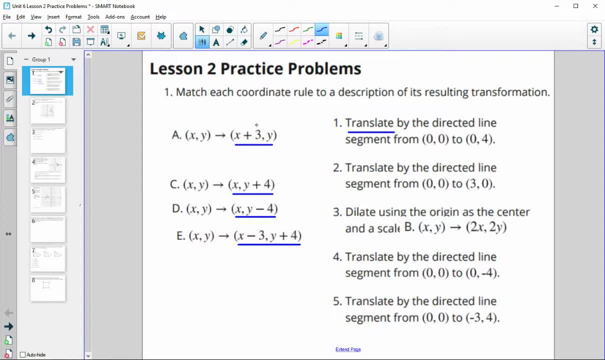 the Y. So this one is moving three to the right and nothing in the Y. So that's going to go to the point three, zero. So that's going to go from zero. like if I plugged in zero, zero here, what I would get back is three, zero. So that's going to go with number two. Okay, you see that zero, zero to. 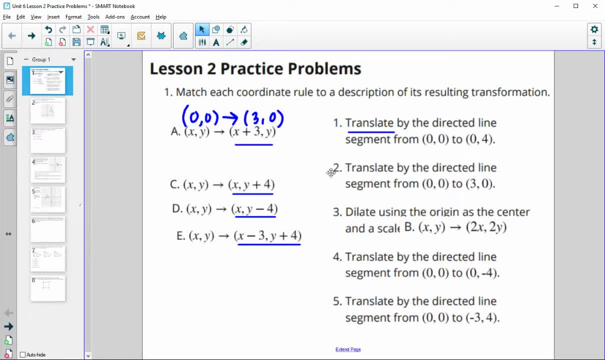 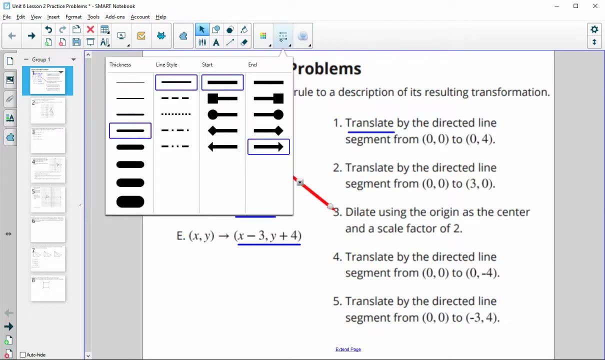 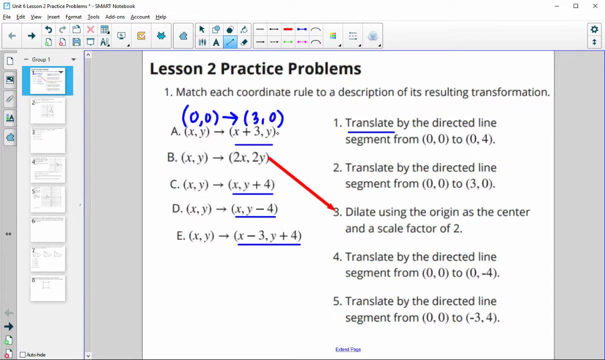 three zero, And so I don't know if it's better to leave these here and draw an arrow, maybe All right. so B went to number three And then A. this zero zero to three zero went to number two. So this one. if we looked at it like this: 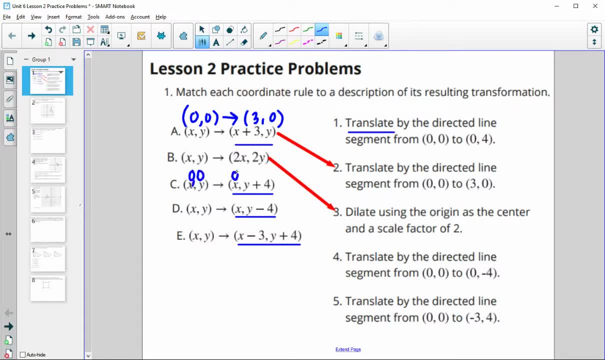 And then we looked at zero zero here. So plugging in zero zero, we would get back zero and we would get back four. So it's going to go from zero zero to zero four. So zero zero to zero four is number one. D is going to go from zero zero to zero negative four. So zero zero to zero negative four is number. 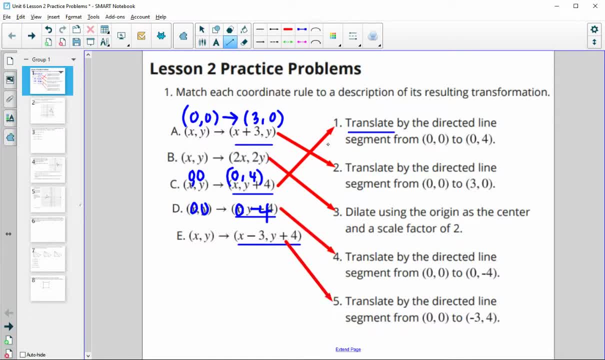 four. and that leaves us with number three: E for number five. So let's clean this up a little bit. So this was C, this was A, this was B, this was D and this was E. All right, draw the image of the triangle under this transformation. So this means: 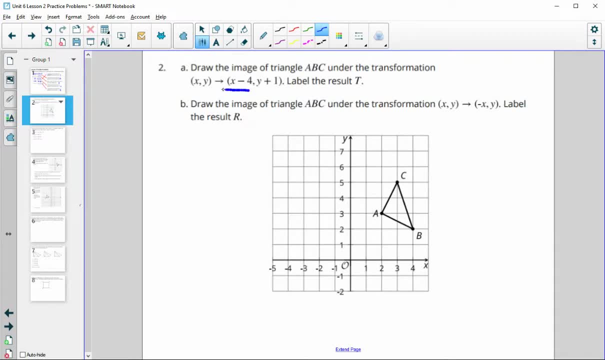 X is going to map to X minus four. That's going to move it to the left four units. and then Y plus one is going to move it up one unit. So every point here we're going to move to the left one and up, or sorry, to the left four and up one. So A is going to go to the left. 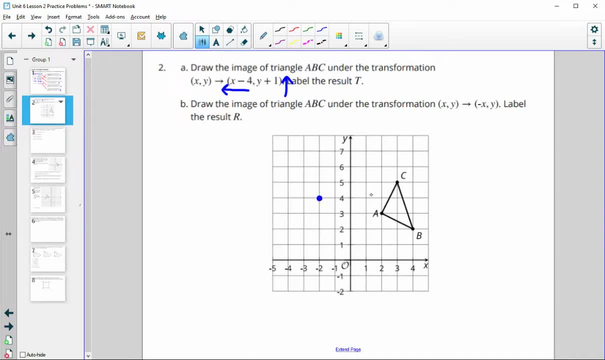 four, one, two, three, four up one, One, two, three, four up one, One, two, three, four up one. And then that's going to give us our new triangle, Triangle- Oops, I don't need an arrow on there. 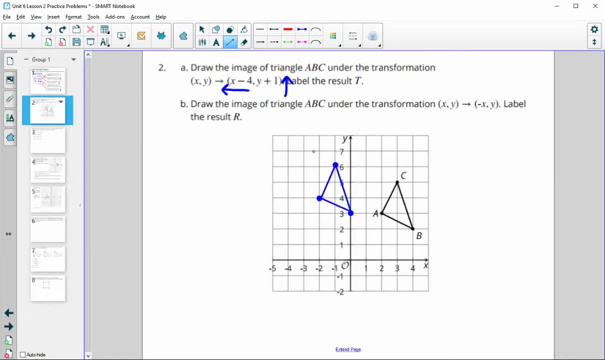 And then we want to label this T. it said, Okay, so that's T, And then draw the image of triangle ABC. So back to the original. under the transformation X- Y maps to opposite X- Y. So we're going to take the opposite. 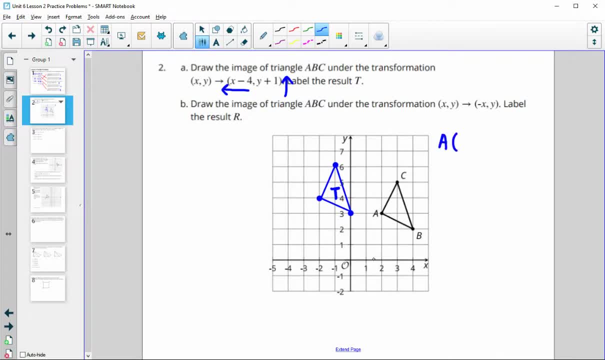 X Y maps to opposite X Y. So we're going to take the opposite. X Y maps to opposite X coordinate. So let me write out these ordered pairs for each point. So A is the point two, three. So that's going to map to the opposite of X. So the opposite of positive two is negative. 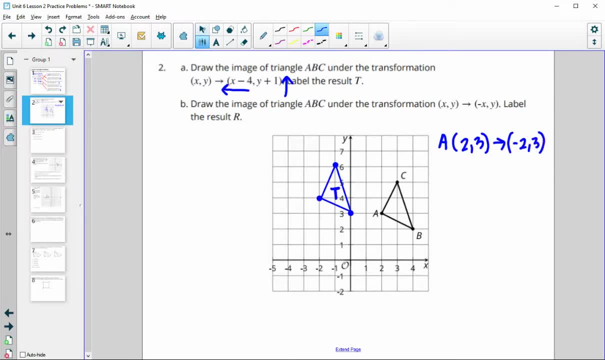 two. And then Y is going to stay the same. Let me change colors here. Whoops, All right. so then point B is the point four: two. So again this is going to map to the opposite. So negative X means opposite of X, not just negative. So that negative out front means 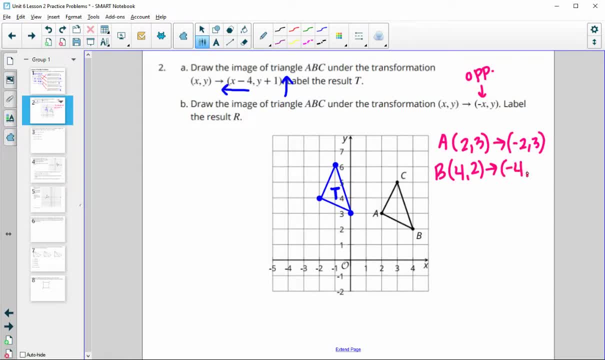 opposite. So four is going to map to negative four, And then the Y coordinate is going to stay the same. C is the point three, five. So again that's going to map to the opposite of three, and then the same Y. 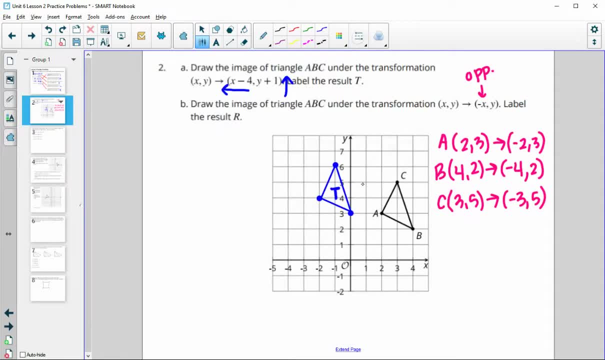 And so what's happening here is we're getting a reflection across the Y axis, since these Xs are just opposite. So, instead of going to two- three, we're going to go to negative two, three. Instead of going to four- two, we're going to go to negative four, two. 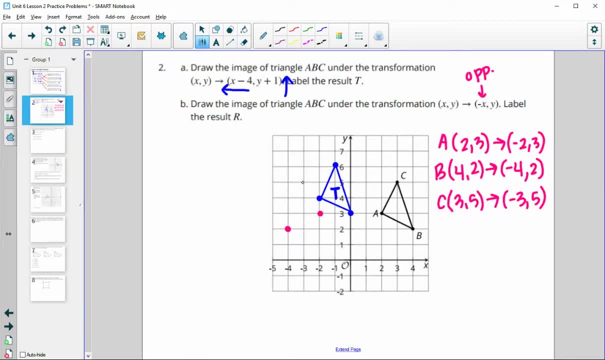 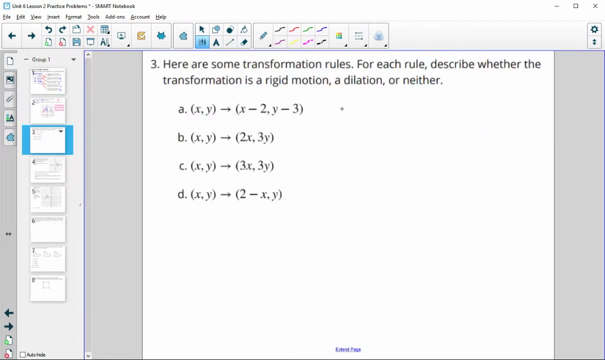 Instead of going to three five, we're going to go to negative three five, And that's going to give us our new image. So it just ends up being a reflection across the Y axis And then label that R Whoops. Here are some transformation rules. for each rule: Describe whether the transformation is. 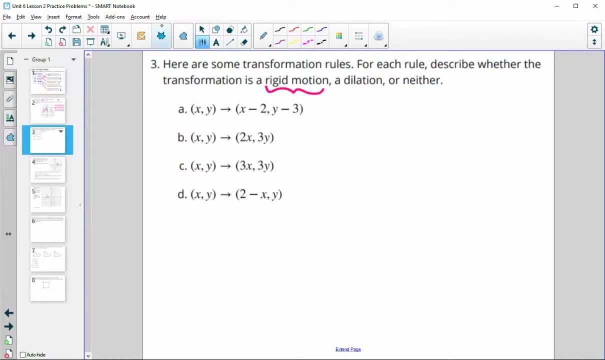 rigid meaning congruent. Okay, So the shape stays the same size. So we're doing a translation, a rotation, a reflection, but the image is staying congruent. Dilation would mean similar or neither. So this one here that you just subtract two, subtract three, So we're just moving to the left. 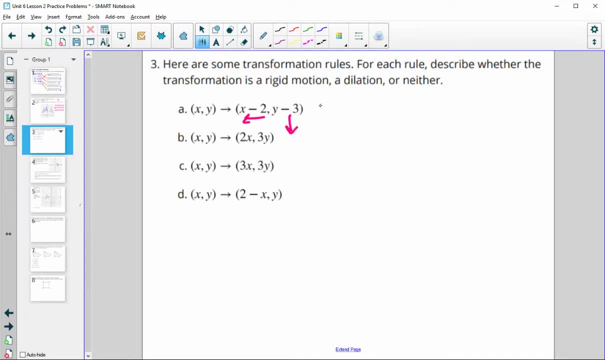 two and down three. So this one is going to be rigid. It's just a translation From zero zero to negative two, negative three. B has multiplication, So that will say that it's going to change size, Since these two numbers are different. so we're not multiplying by the same scale factor. 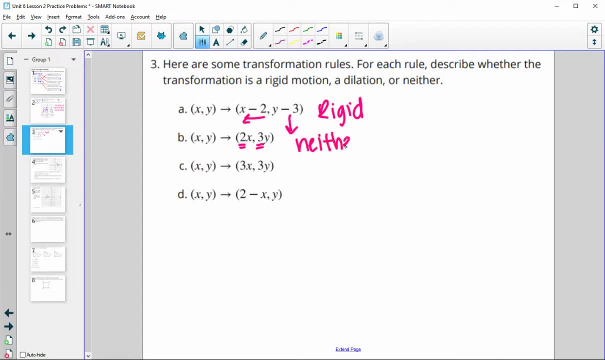 this one is going to be neither, Because it's going to get two times wider but three times taller. So it's not going to be similar Versus C. since these are the same, it's going to be a dilation. So these are going to stay similar. The scale factor is three. 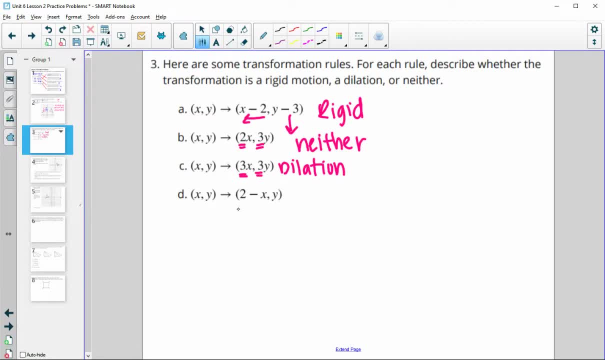 This next one. okay, kind of interesting the way this is written, We could rewrite this X part as negative X and then plus two. So this one is doing kind of a reflection and a translation, because we've got that negative or the opposite of the X. 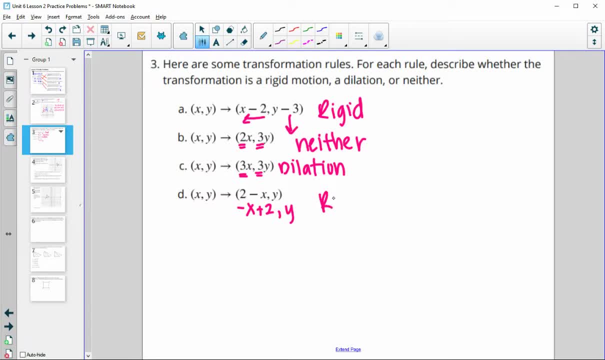 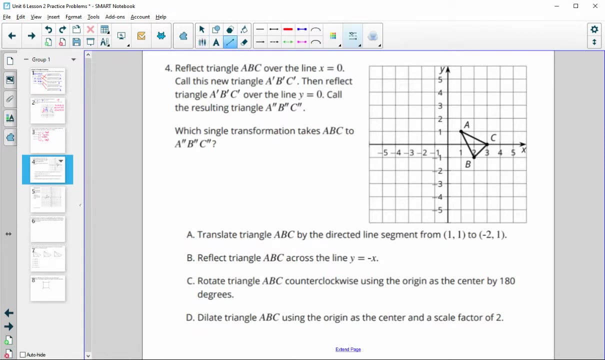 And we're moving to the right. So this one is still going to be rigid because it's just a translation and a reflection together. All right, reflect: triangle ABC over the line X equals zero. So let's plot the line X equals zero so we can see it. So X equals zero is the Y axis. 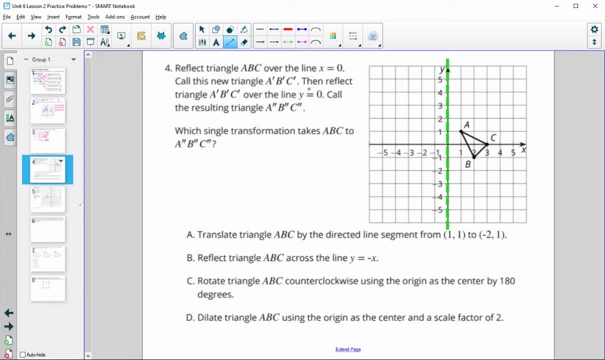 And call the new triangle A prime, B prime, C prime. then reflect that over the line Y equals zero, All right. so this one, the green one, is X equals zero, Okay. and then the pink one is Y equals zero. So Y equals zero is the X axis. 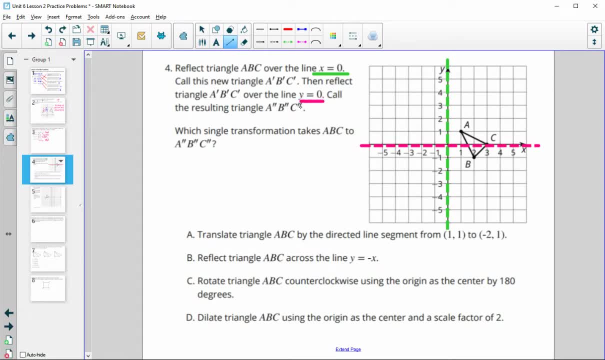 And call that A double prime, B, double prime, C, double prime, Then what single transformation would take ABC to A double prime, B, double prime, C, double prime. So let's reflect over the green line first. So A is one to the right, So A prime will be one to the left. 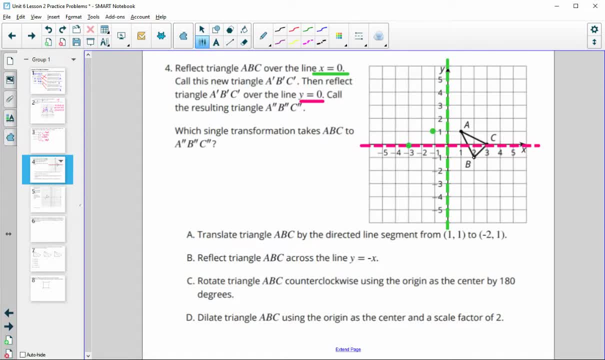 C is three to the right, So we'll go three to the left. B is two to the right, So we'll go two to the left. And here's our whoops. here's our new image. Now we want to take this image and we want to reflect it over the Y axis. 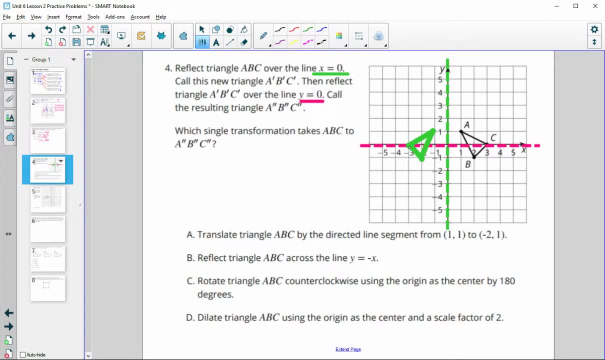 Okay, so now we're going to flip over the Y, or sorry, the X- axis, So this point is going to stay. This one is one above, So now it'll be one below. This one is one below, So now it will be one above. 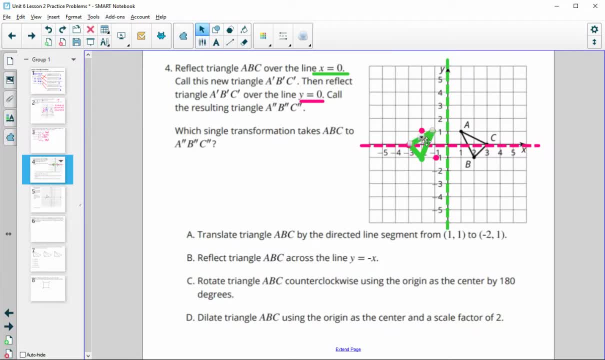 And we'll get our new shape here. So actually I'm going to do a little bit of a flip here. I'm going to delete out these so we don't get lost with those anymore. So here's our new triangle. So what one motion would have taken us from this black one to this pink one? 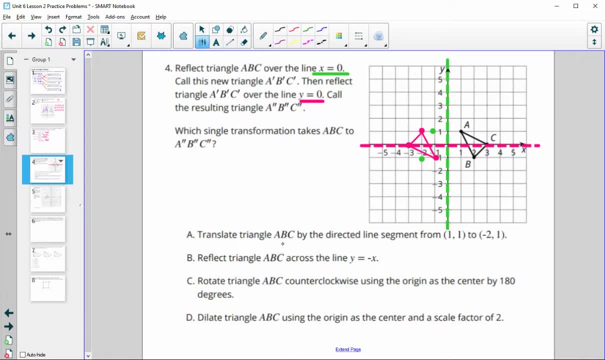 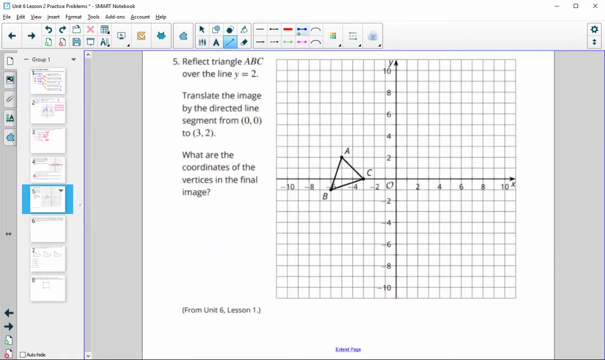 And so that looks like it's going to be a 180 degree rotation. So rotate the triangle clockwise using the origin: 180 degrees. All right, reflect the triangle over the line Y equals two. So let's plot: the line Y equals two. 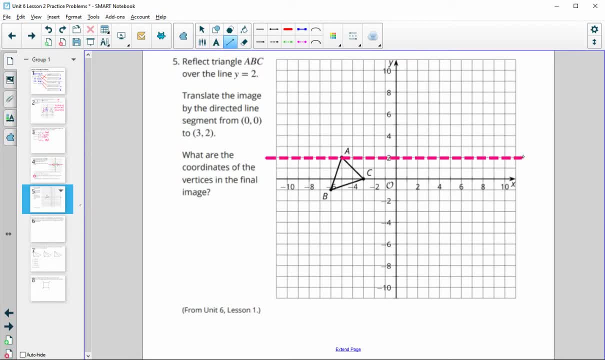 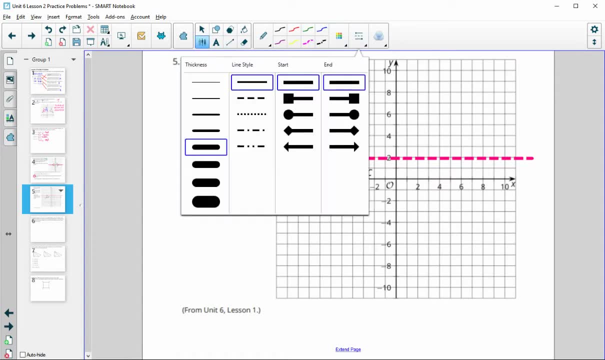 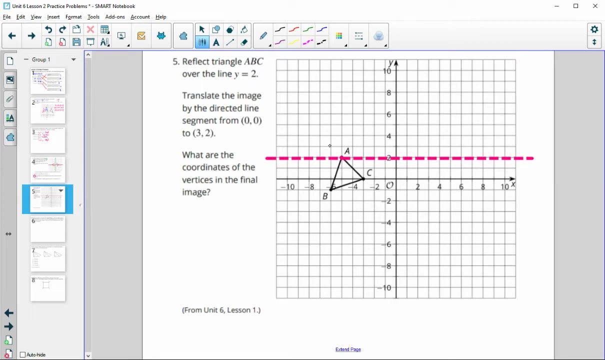 So a. Y equals line is a horizontal line, So Y equals two is right here. So let's reflect the triangle first over that line. So A is going to stay in place. B is three below. So A is going to stay in place, B is three below. 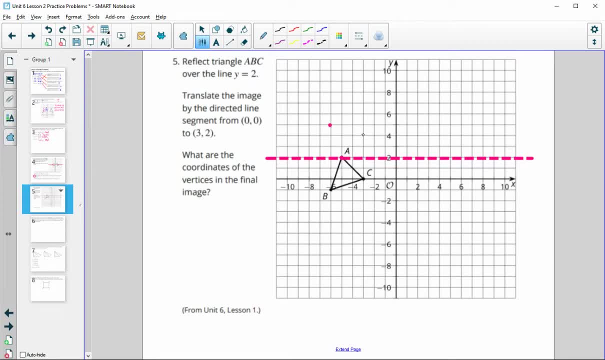 So B prime is going to be three above, C is two below, So C prime is going to be two above, And that will get us our new triangle here. So let's label those. So A and A prime are the same: C prime here, B prime here. 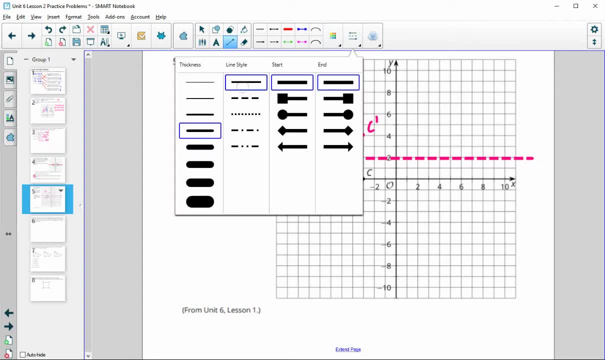 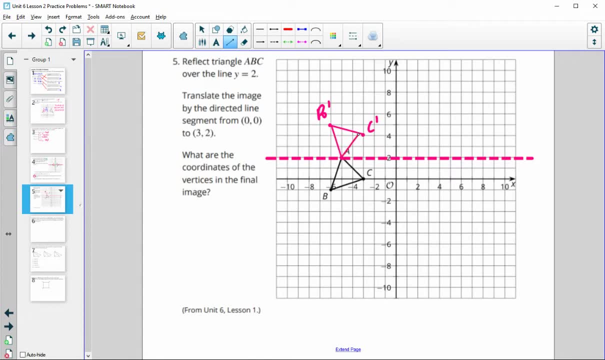 And then connect them. So here's our new triangle. Then translate the image by directed line segment from 0, 0 to 3, 2.. So this is going to be 3 to the right and 2 up. So we're going to take every point and move it 3 to the right. 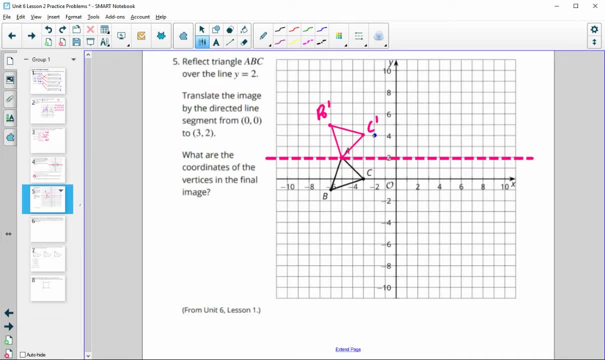 So 1, 2, 3 and 2 up, 1, 2, 3, 2 up, 1, 2, 3, 2 up And get our new image here. So let me connect these again. 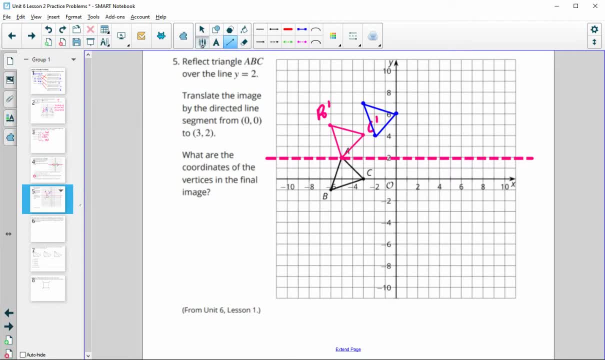 And so this is our C double prime was here. This one was A double prime, This one was B double prime. So what are the new vertices? So A double prime is, at what Negative? 2, 1,, 2,, 3,, 4.. 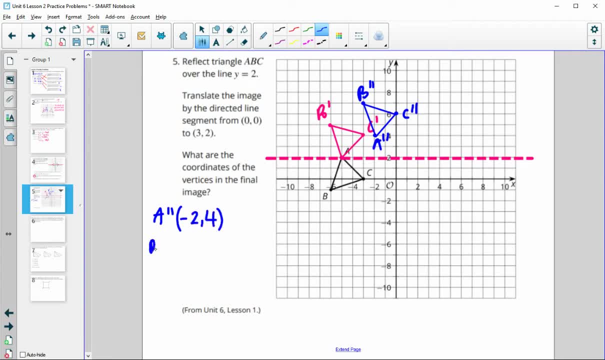 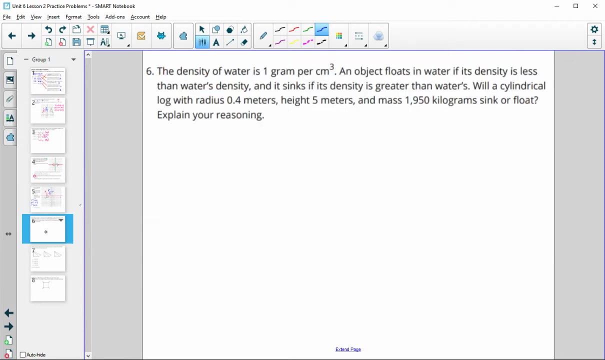 So negative 2, 4.. B double prime is at one, two, three, seven. so negative three seven. and C prime is at zero six. C double prime is at zero six. all right, density is mass divided by volume. so in this problem it tells you that the 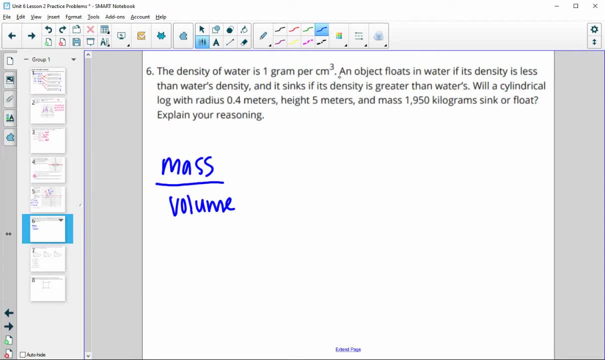 density of water is one gram per cubic centimeter. if the density of an object is less than that, it will float. if it's higher than that, it will sink. higher than one it'll sink. so will a cylindrical logs. we've got a cylindrical log, so we're gonna be doing volume okay. so remember that will be. 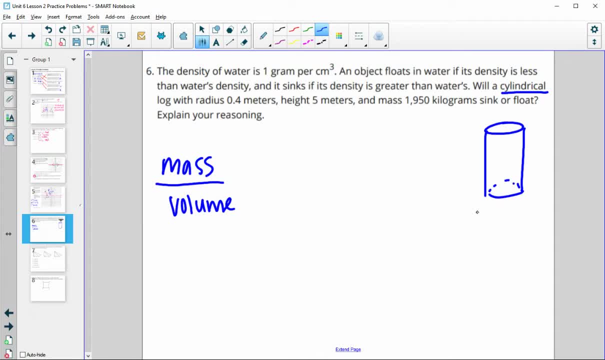 important that it's a cylinder because the volume will equal area of the base times. the height has a radius of 0.4 meters. okay, so the radius of this is 0.4 meters and the height is 5 meters and its mass is one thousand nine hundred five. 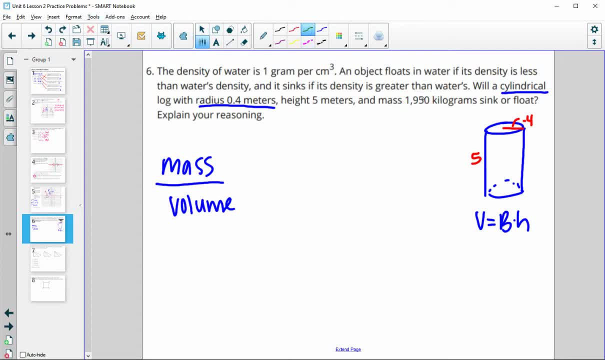 milligrams on that. the area of the base square is the radius of that area. so going with a festivals case, these graphs are given right. here we have: the mass here is 1,950 kilograms. is it gonna sink or is it gonna float? so the mass here is 1,950. so now we just need the volume. so we'll need to do area of the base times the height. so the way that we do the area of the base would be pi times the radius squared. so pi times 0.4. 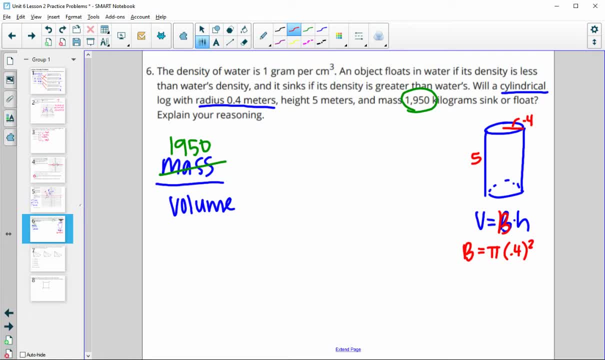 squared, and so 0.5 is 1.7. all right, this is vale 2 and 1.2 and 1.2. all right, we got this all right. it's so over 10, 0.4 times 0.4 is 0.16.. So we'd have 0.16 pi for the area of the base. 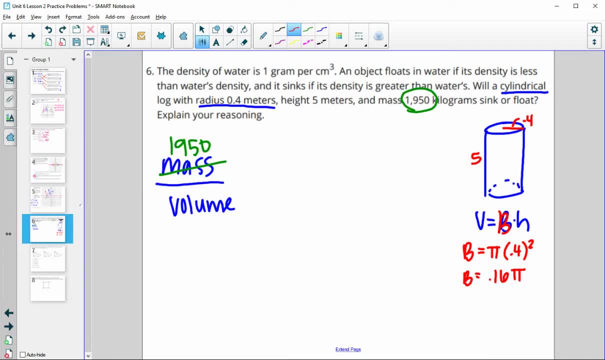 So then, if we multiply that 0.16 times pi, we get the area of the base is 0.502654, blah, blah, blah, And then the height of this is five. So for volume we'll multiply those together. So 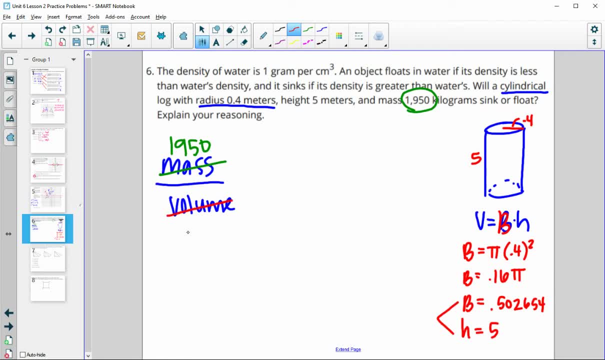 point. multiply that decimal times five and we get the volume is 2.5.. And let's see 0.45 meters. Okay, And then the mass is kilograms. All right, So then 1950 divided by 2.5.. 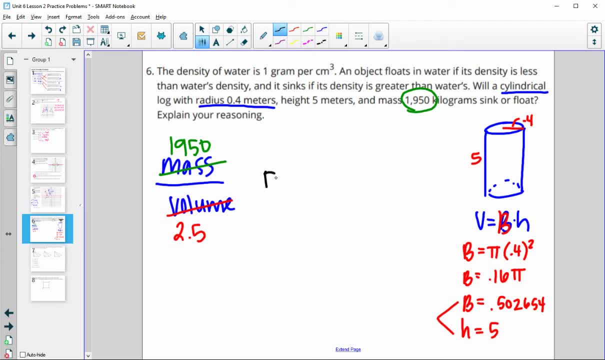 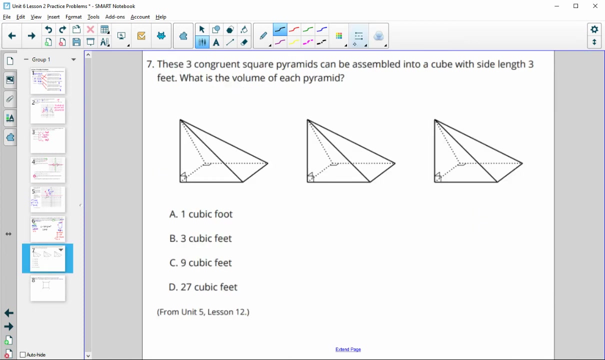 2.5.. So the density of this is going to be 780 grams per cubic centimeters. So that is much higher than one. So this is going to sink All right. Number seven: These three congruent square pyramids can be assembled to a cube. 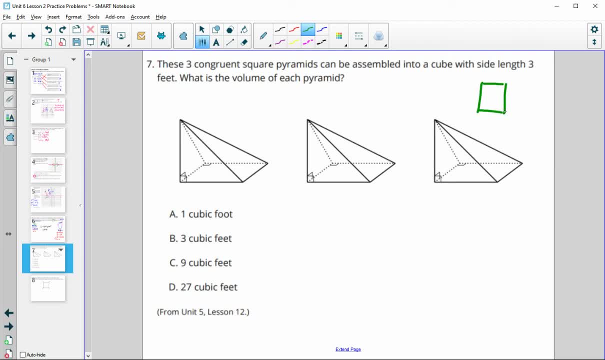 with side lengths of three. So, remember, a cube is a square. So this is going to be a cube. So this is going to be a cube Has all of its lengths being equal. Okay, So all of these are three. What's the volume of each pyramid? So to find the volume of a cube, remember, you just take a side. 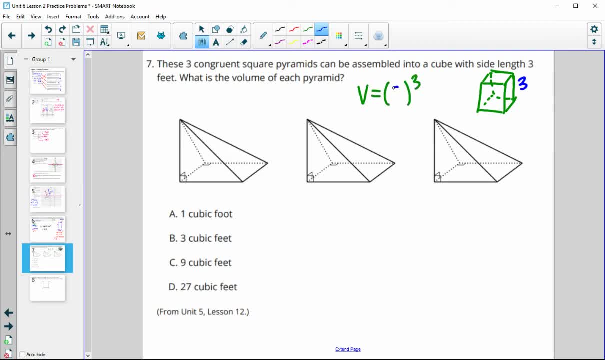 cubed. So we just take this side and cube it. So the volume of this cube is going to be 27.. And then each of these three pyramids is identical. okay, so all three of these have the same exact volume. so we'll just divide this by three to 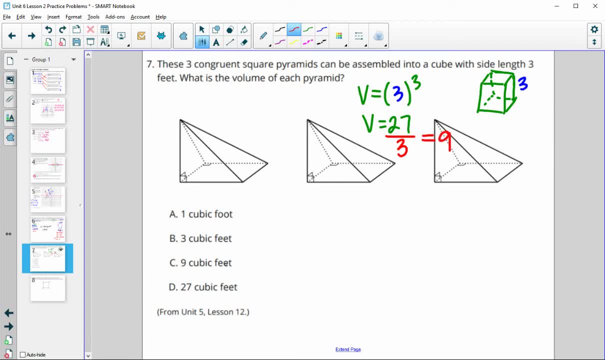 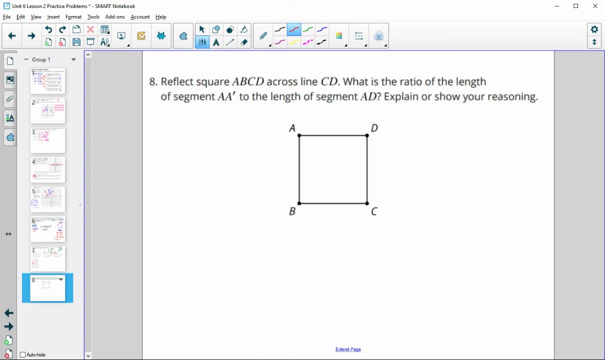 figure out how big each one is. so 27 divided by three gives us nine cubic feet. then number eight says reflect square a, b, c, d, a long line cd. so we're gonna reflect it um over cd. so here's the line cd. so we're gonna reflect it over here. 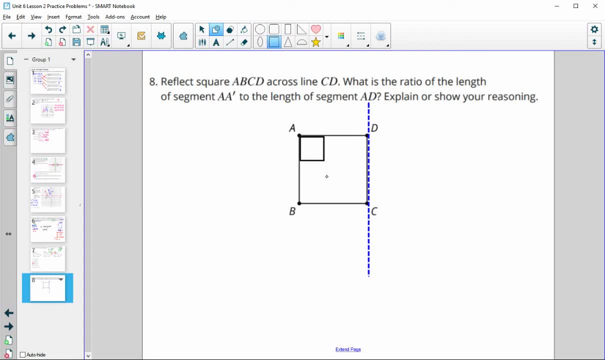 whoops, that's a circle. all right, so if we reflect this um square over that line, you're just gonna end up with the square here. c and c prime, d prime would stay in the same spot, and then here would be a prime, b prime. um, what would be the ratio of the length of segment a to a prime? okay, so here's a to.